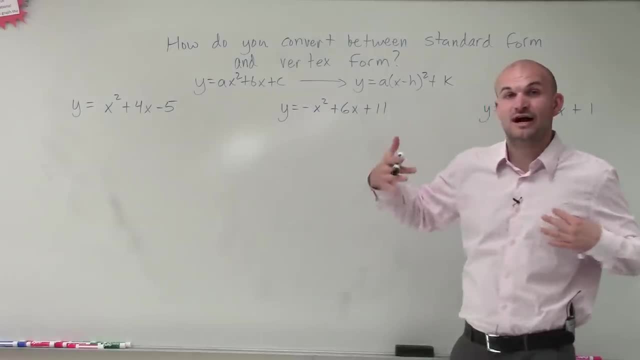 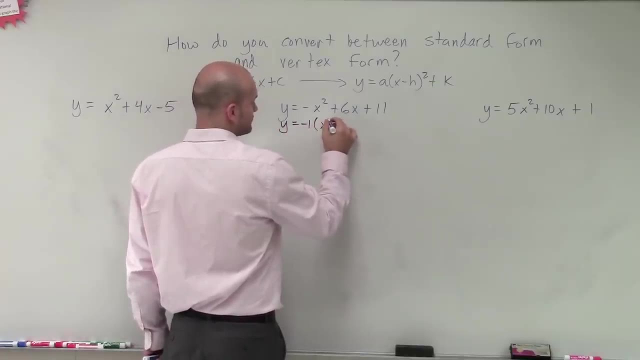 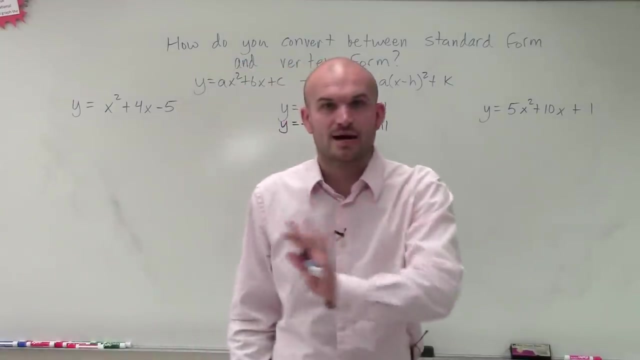 to have to do is factor that out. Now I'm completing the square, I only like to factor it out of the first two terms. So I have: y equals a negative one times x squared minus six x plus 11.. All right, Now I'll talk about again completing my perfect square and what we're. 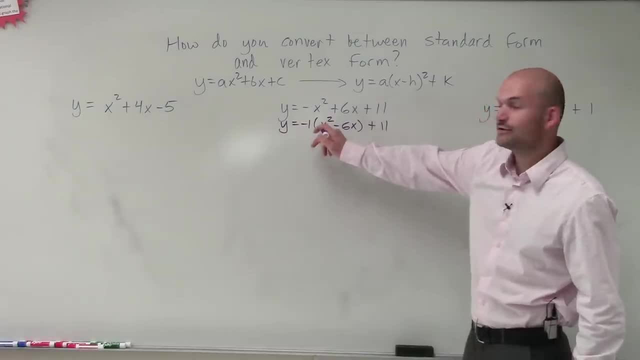 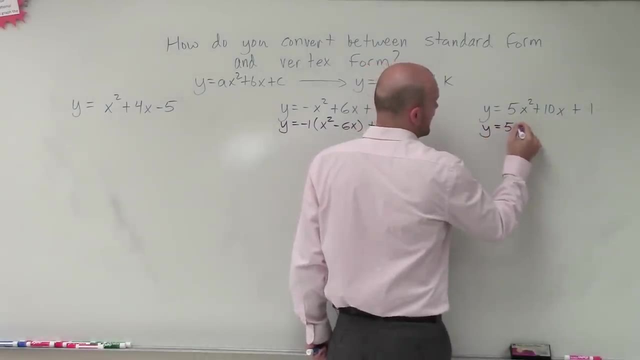 going to do. But as long as my a now is equal to one, I'm all set Over here. I have to factor out a five. So I'll factor out a five. So I have y equals five times x squared plus two x. 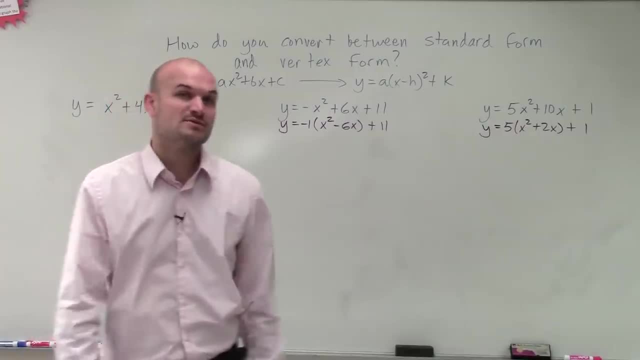 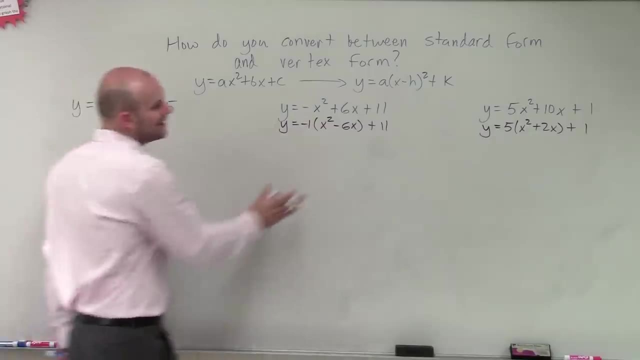 plus one. Now again, I'm only factoring out of these first two terms because I'm going to show you what I'm going to do is I'm going to now create All right, And what we're going to do is we're going to look at only my quadratic and my linear term. So right now, those are a binomial. 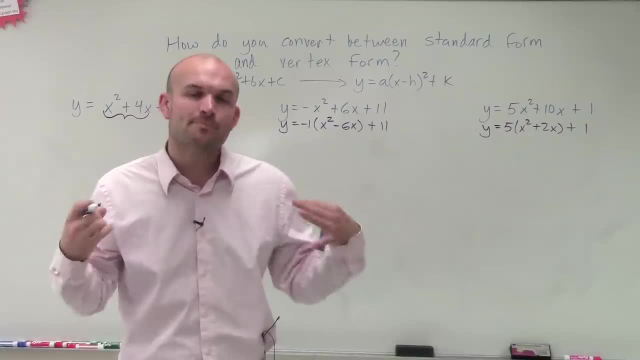 And what I'm going to do is I'm going to take those terms and create, make them into a perfect, square trinomial, And I'll show you how. So to do that. what we're going to do is we're going to 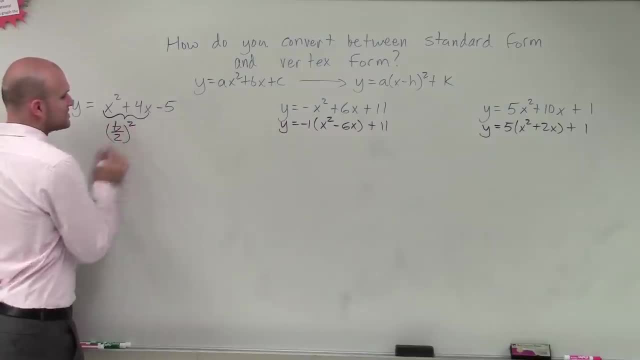 take b divided by two and then square it. So in this case, my b. if we have a b, we're going to take b divided by two and then square it. So in this case, my b- ax squared plus bx plus c, b is my coefficient of my linear term, So that's going to be four. 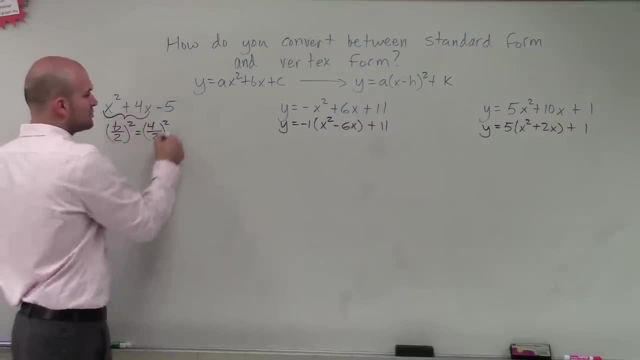 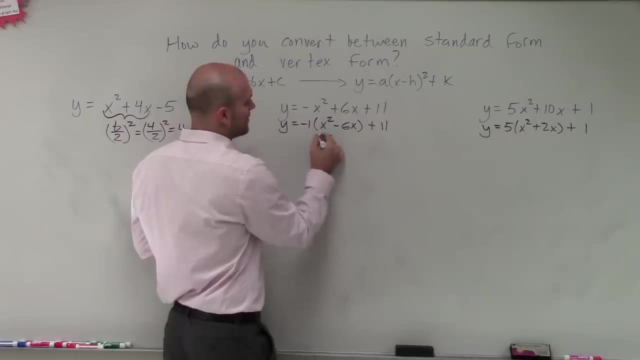 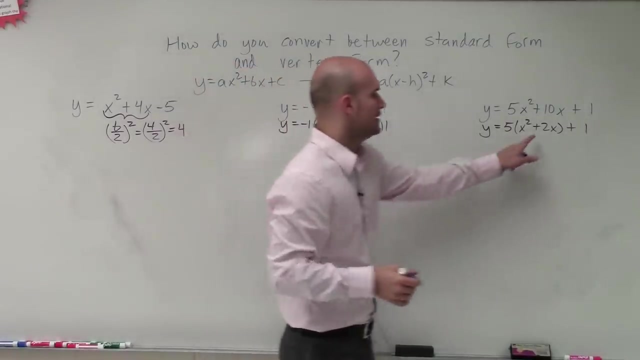 divided by two squared Well. four divided by two is two. Two squared is equal to four. Here my b divided by two is going to be negative. six divided by two squared Well, negative. six divided by two is negative. three, Negative. three squared equals nine. Here, 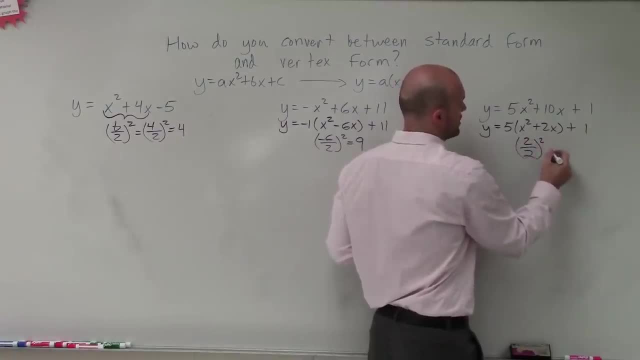 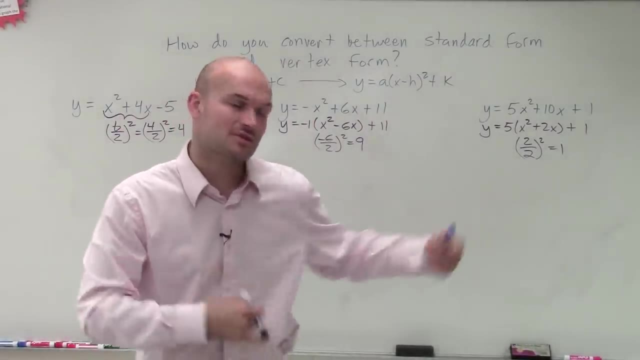 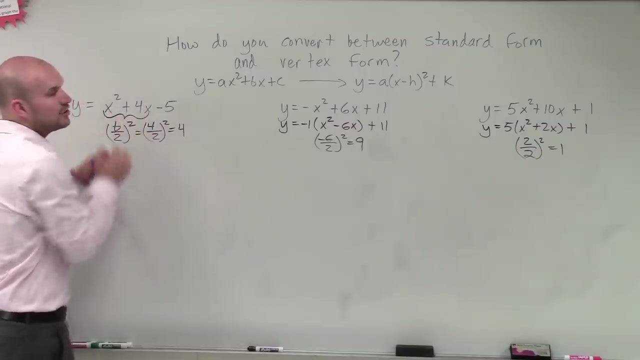 I'm going to take two divided by two and then square it, And that equals one. So now what I'm going to do is that is my value. that completes my perfect square. So what I'm going to do with each one of those values is: I'm now going to add it to my other two terms, And what that's going to. 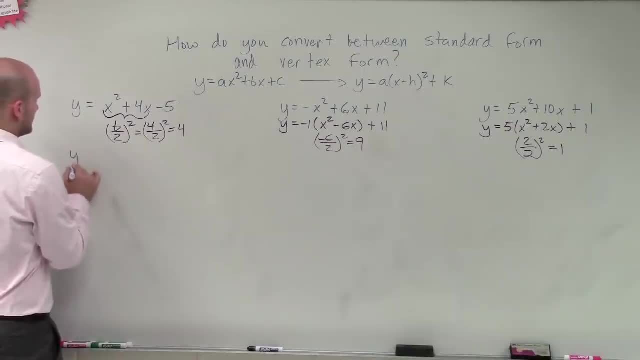 do is that's going to now create a perfect square trinomial. So let's go ahead and write that out now. So when I add that in there, so I have x squared plus 4x plus four. Now what I've done is: 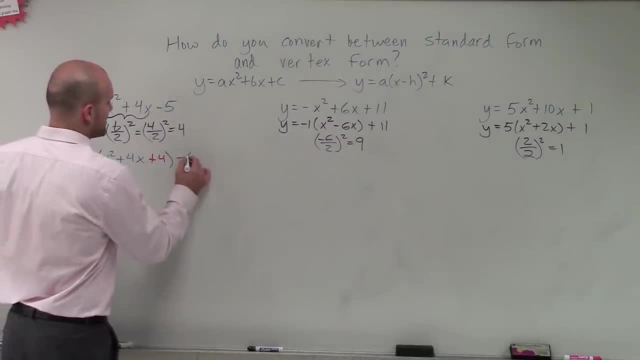 I have created a perfect square trinomial and then I'll just have minus 5.. Now I'll come back and I'll explain something in a second. So here I'm going to add 9, now inside the parentheses. 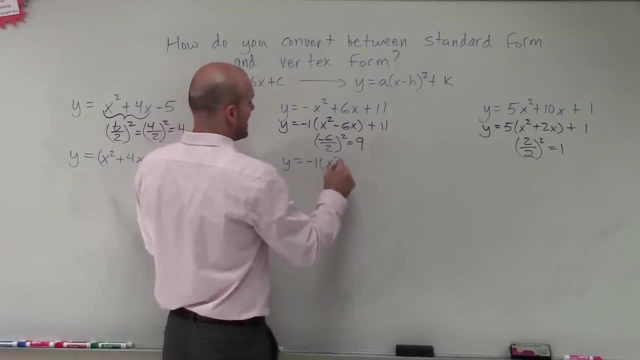 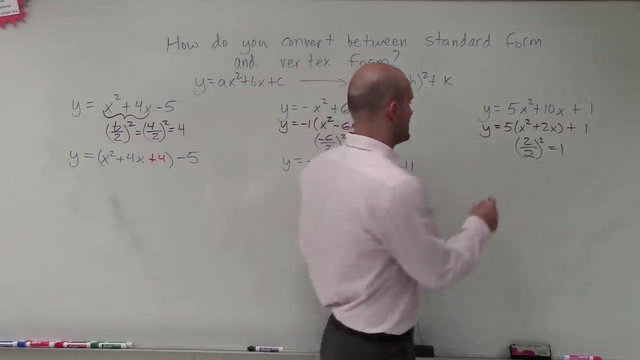 So I'll have y equals negative x squared minus 6x plus 9 plus 11.. And then over here I'll add 1 inside the parentheses, So I'll have y equals 5 times x squared plus 2x plus 1 plus 1.. 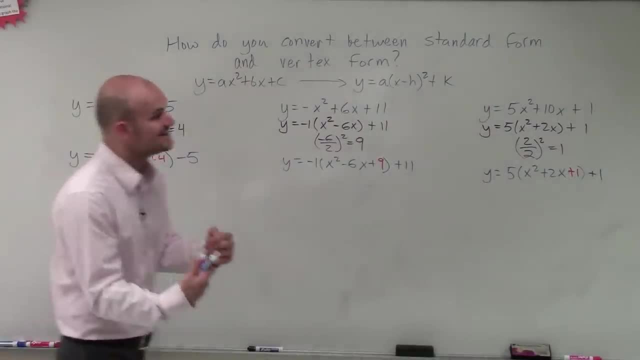 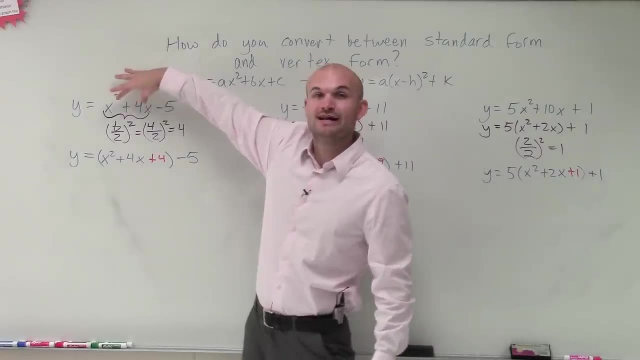 OK, so notice how everything else is staying the same. The only thing I did is I took my middle value divided by 2, squared it and then added it to my quadratic and my linear term to create a perfect square trinomial right. 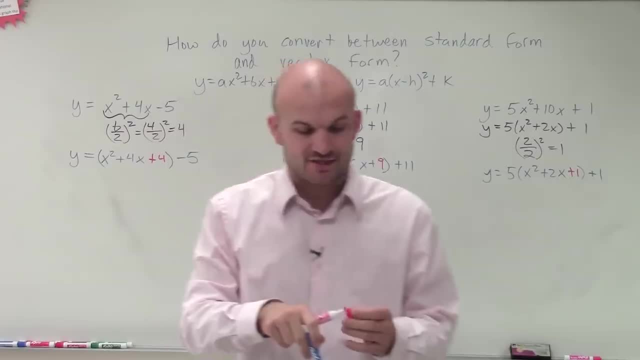 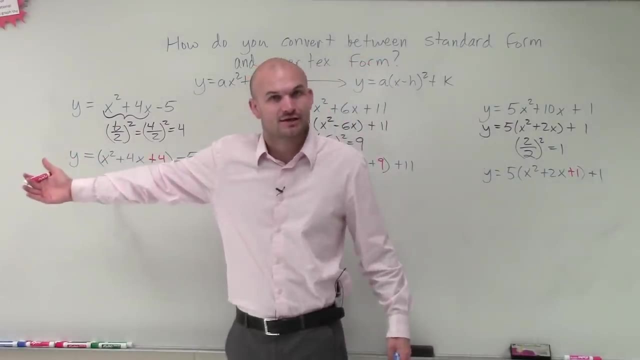 OK, now, adding this number is great, but you've got to look at this and we have an equation going on. When we have an equation, you just can't add numbers to one side of the equation without adding them to the other side of the equation, right? 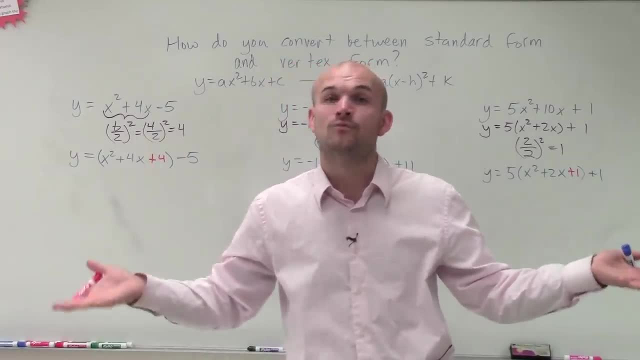 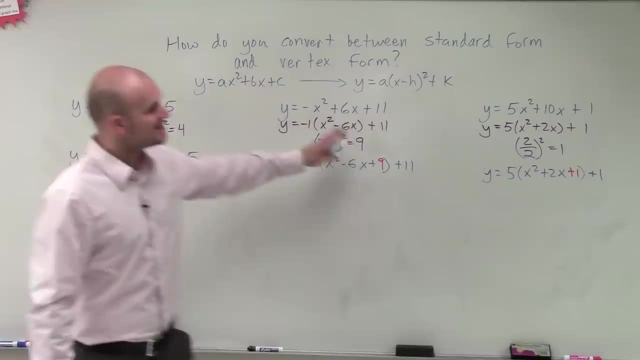 If I have an equation, if I add 1 to the left side, I have to make sure I add 1 to the right side. So that was about using our properties of equality. So right now you can see all to the right side. 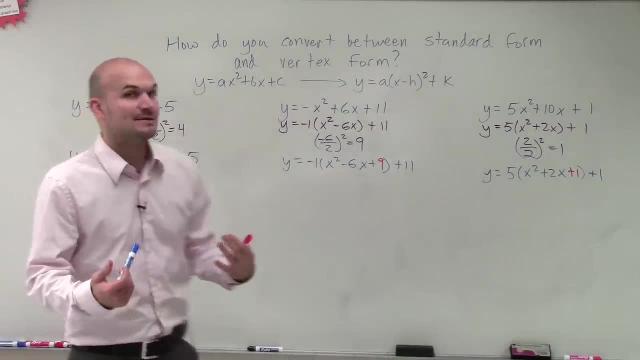 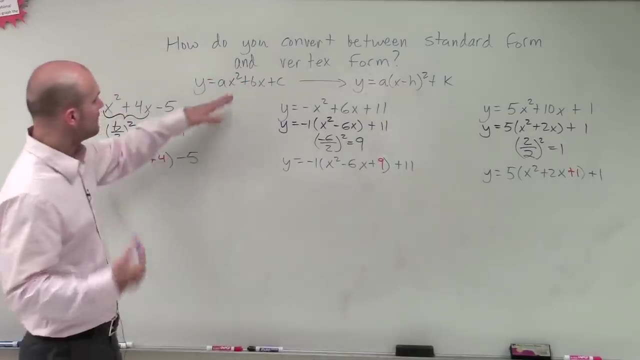 I'm adding a value Now, when solving, a lot of times, what we like to do is we like to add it to the other side as well, because that's going to be your equality. However, when I'm trying to convert it from one form, 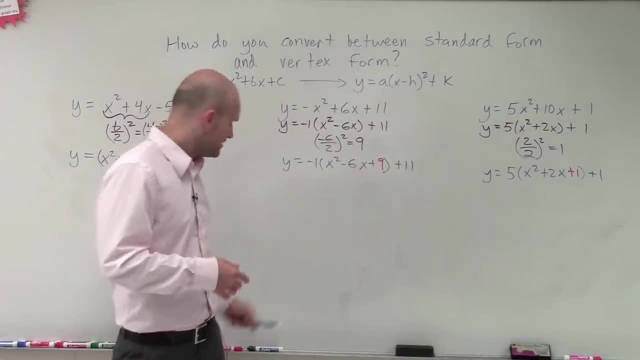 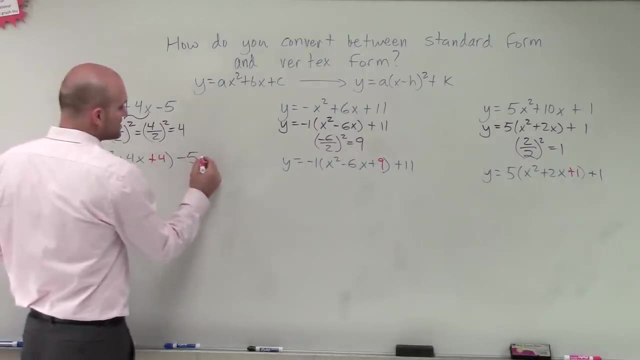 to the next. I'm still solving each value for y. So, rather than adding the same value to both sides, what I'm going to do is I'm going to add the 4 to the right side, but then I'll just simply subtract. 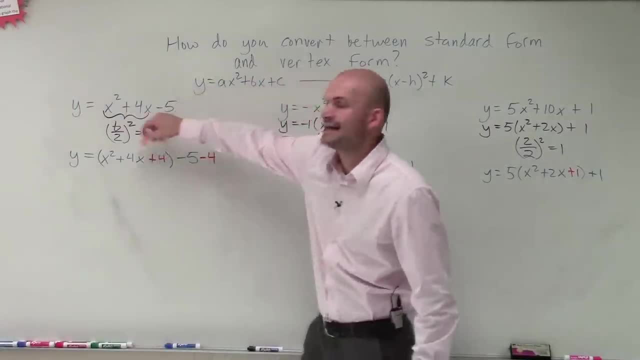 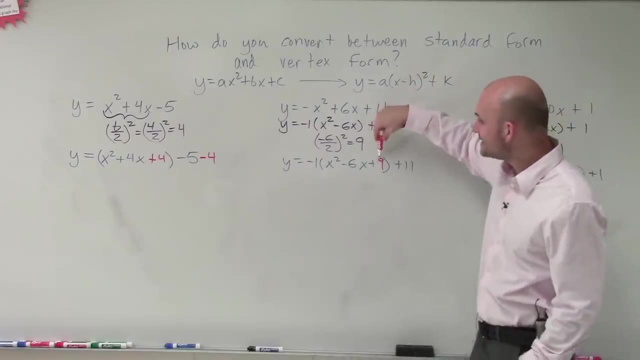 it on that side as well, The difference being is one value I added inside the parentheses and the other value I'm adding outside the parentheses. Well, that's very important, because when I add 9 inside the parentheses, you notice that this 9 is being multiplied by negative 1.. 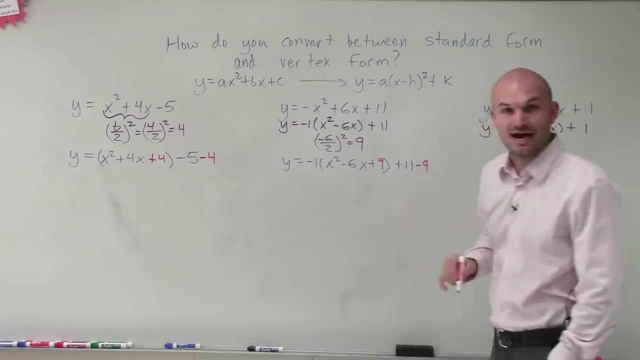 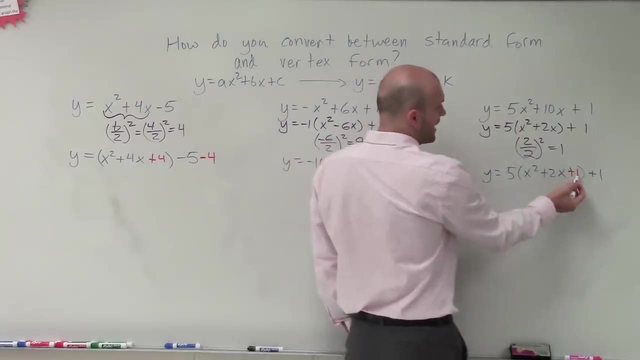 So when I subtract the 9.000.. outside the parentheses, I have to make sure I also multiply that by a negative 1. Over here when I add this 1,. so now I'm going to subtract 1, notice that the 1 inside the parentheses is. 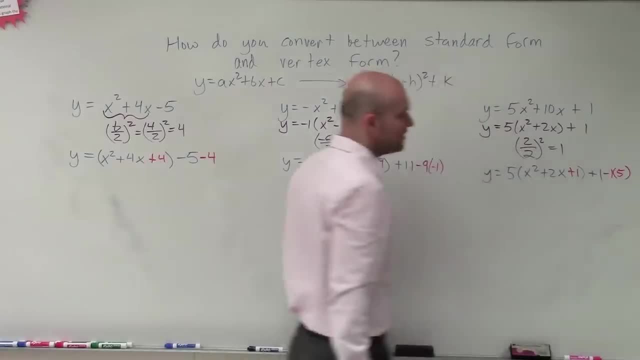 being multiplied by 5.. So I need to multiply this 1 by 5 as well. All right, So why are we working with the perfect square trinomial? Why do we want this trinomial, Or what is a perfect square? 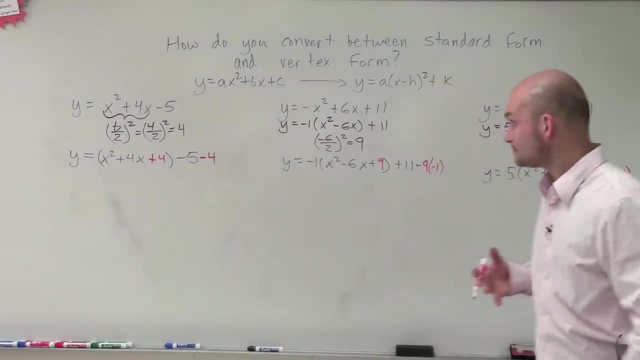 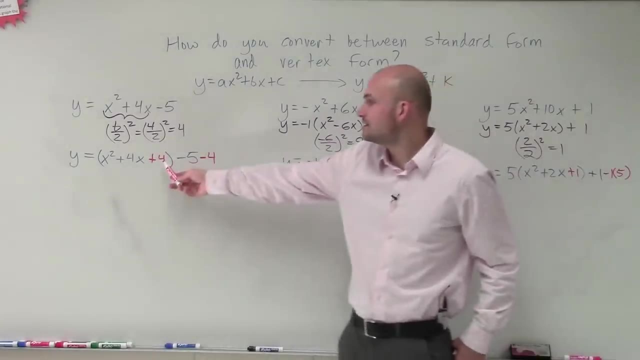 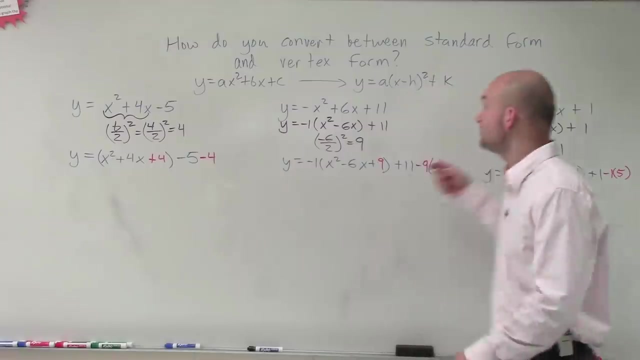 trinomial. A perfect square trinomial is when we have the exact same values multiplied to give us our c value, but then add up to give us our b value. So what all these perfect square trinomials can be factored into are binomial squares. So now I just simply need to say: all right. 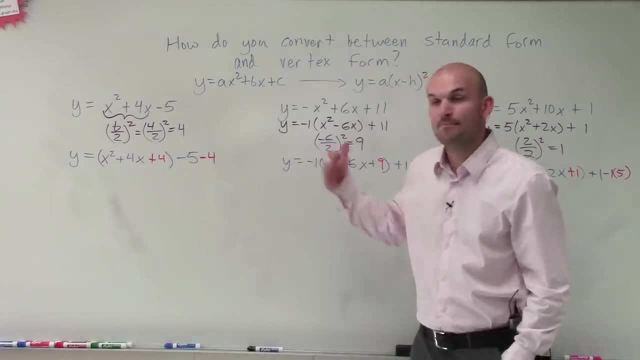 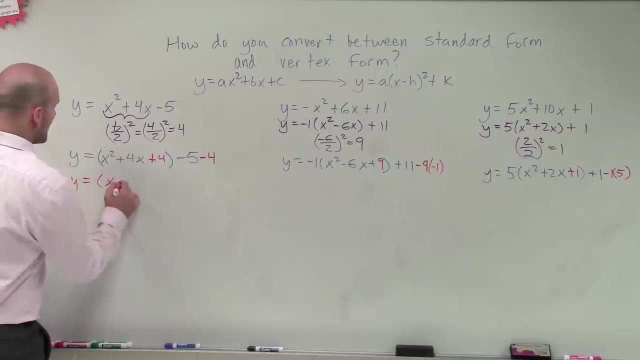 what two numbers that are exactly the same. multiply to give me 4 and then add to give me 4? And we can say that my final value is going to be: y equals x plus 2 squared, And then I can just combine negative 5 minus 4. 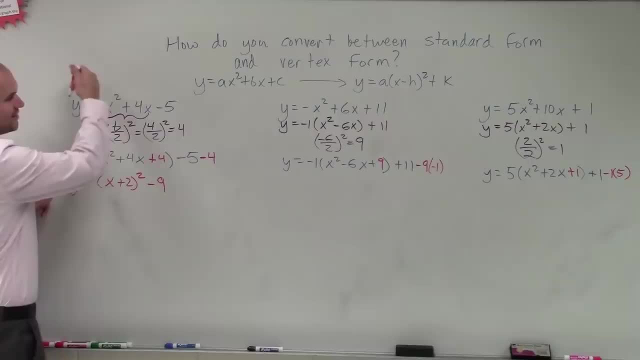 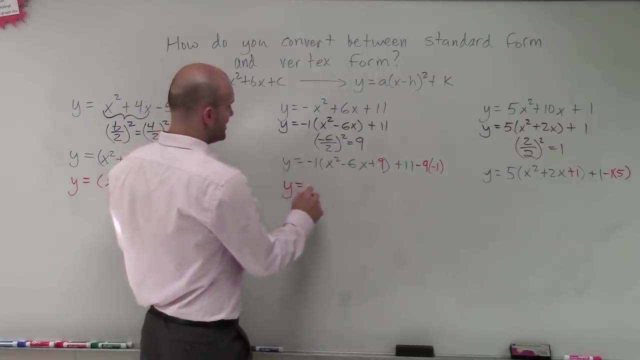 is a negative 9.. Now I have taken this equation from standard form all the way into my vertex form. Here, when I write this, I have y equals negative. I don't really need to write the 1.. So now I see what two numbers that are exactly the same. 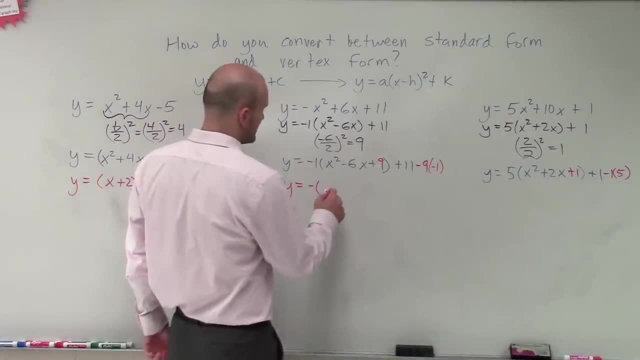 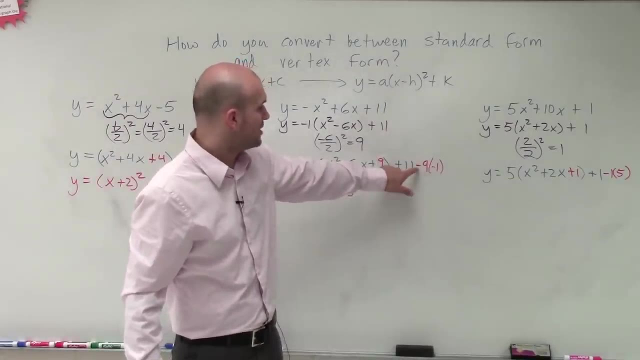 multiply to give me 9 and add to give me negative 6.. Well, that's going to be x minus 3 squared. Notice how I'm always getting this binomial squared. Then I look at this. I say negative 1 times negative. 9 is positive 9.. 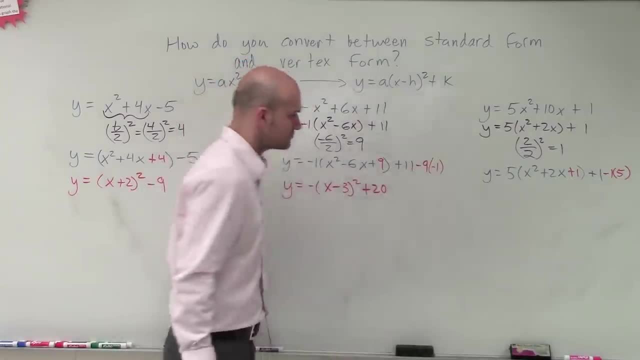 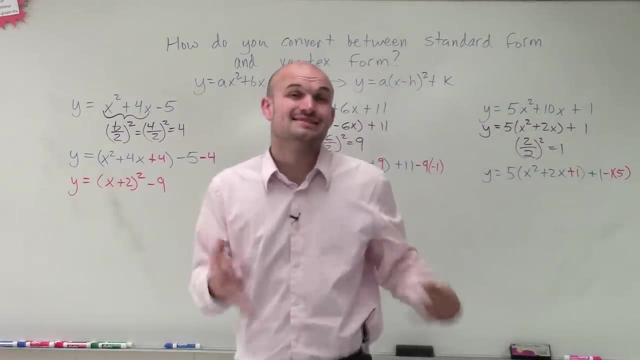 Positive. 9 plus 11 is 20.. And there you go. Now my equation is in vertex form Over here. I say: what two numbers that are exactly the same? right, Because a perfect square trinomial always gives you a binomial squared. 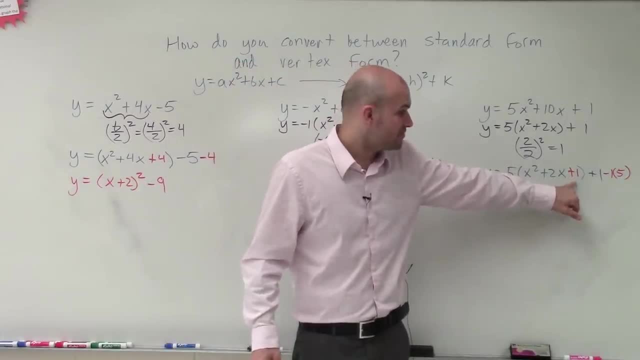 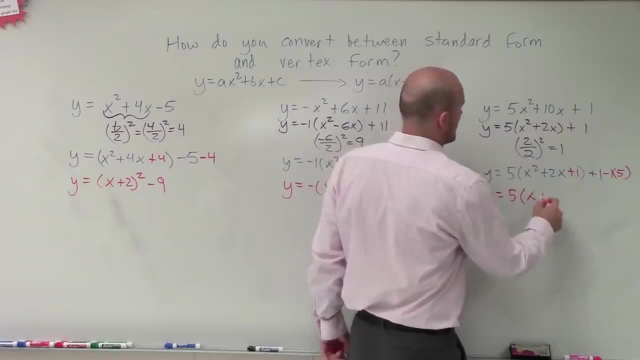 What two numbers that are exactly the same give me 1,. multiply to give me 1, and add to give me 2? Well, that's going to be x plus 1.. And x plus 1.. So I say y equals 5 times x plus 1 squared. 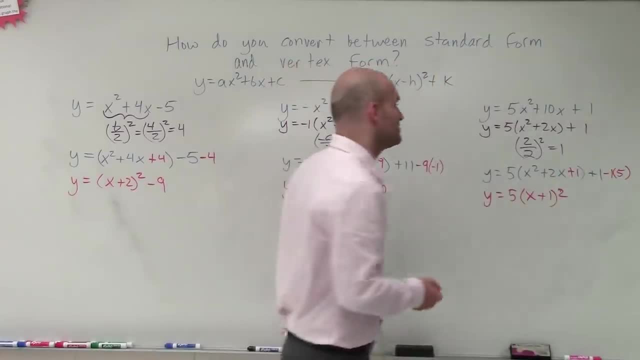 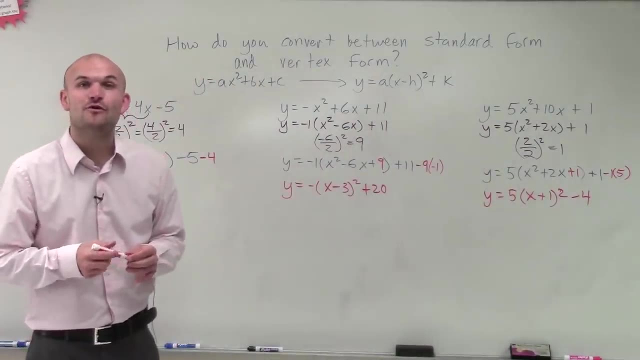 And then 5 times negative. 1 is negative. 5 plus 4 is negative 4.. Or plus 1 is negative 4.. So there you go, ladies and gentlemen. That is how you convert between standard form and vertex form. Thanks, Thank you. 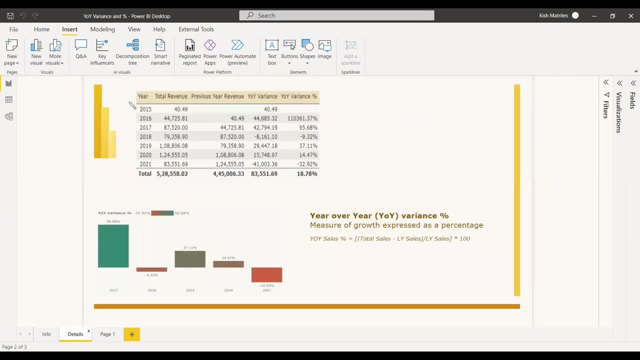 YOY variance percentage. So when you go to the detailed view, you can see these are the years we are having and these are the revenues we are having with respect to these years, and you can get the previous year's revenue. Of course, the previous year's revenue will be the just minus.